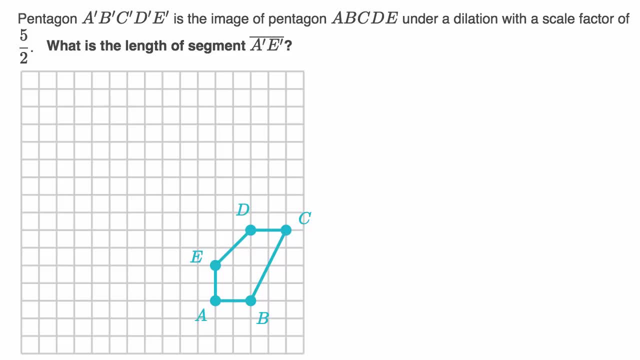 Let's do another example. So we are told that pentagon A, prime B, prime, C, prime, D, prime, E, prime is the image and they haven't drawn that. here is the image of pentagon A, B, C, D, E under a dilation. 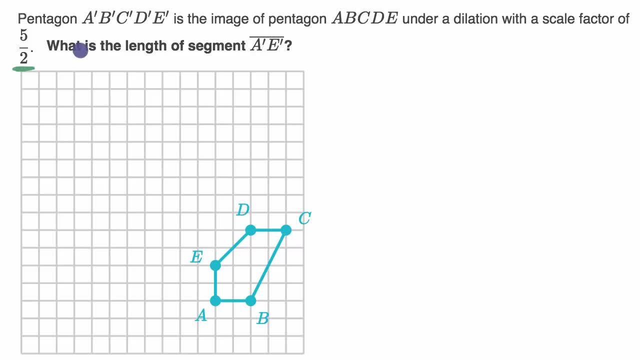 with a scale factor of 5 1⁄2.. So they're giving us our scale factor. What is the length of segment A? prime, E, prime. So, as I was mentioning while I read it, they didn't actually draw this one out. 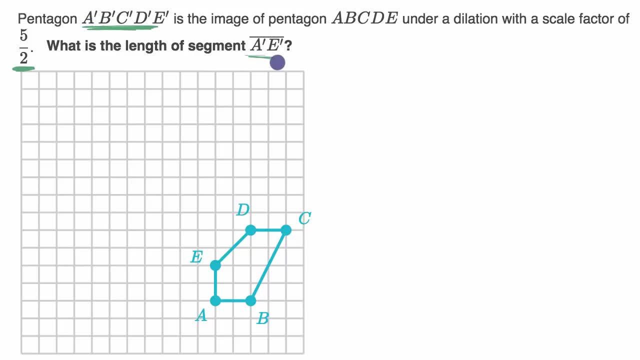 So how do we figure out the length of a segment? Well, I encourage you to pause the video and try to think about it. Well, they give us the scale factor, and so what it tells us? the scale factor is 5 1⁄2.. 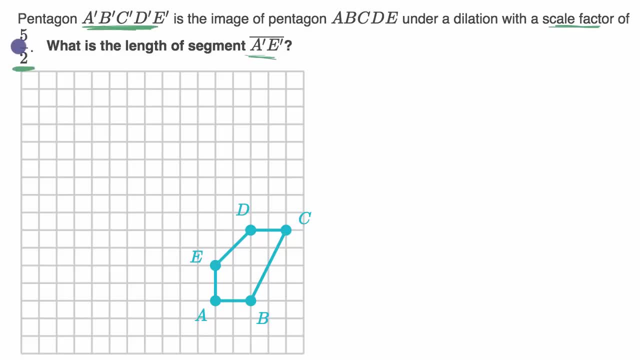 That means that the corresponding lengths will change by a factor of 5 1⁄2.. So to figure out the length of segment A, prime, E, prime. this is going to be. you could think of it as the image of segment AE. 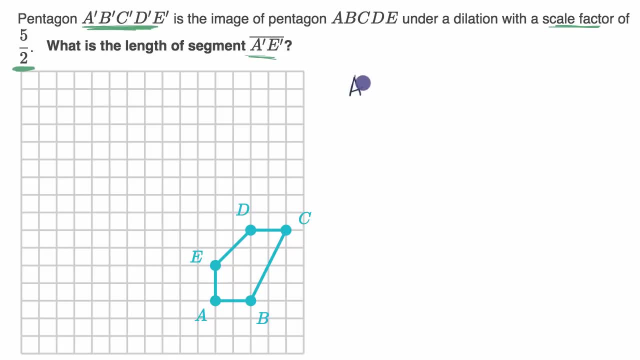 And so you could see that the length of AE is equal to two, and so the length of A prime, E prime- is going to be equal to AE, which is two times the scale factor times 5 1⁄2.. 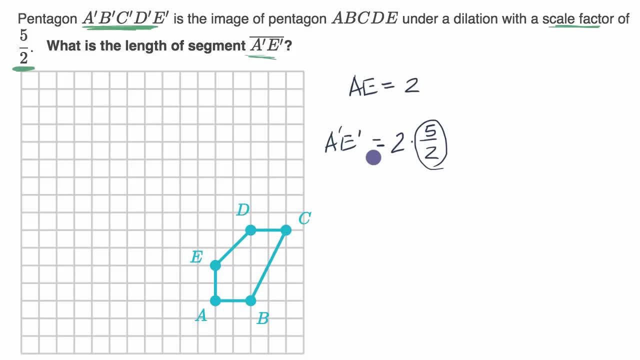 This is our scale factor right over here. And, of course, what's two times 5 1⁄2?? Well, it is going to be equal to five, five of these units right over here. So in this case we didn't even have to draw. 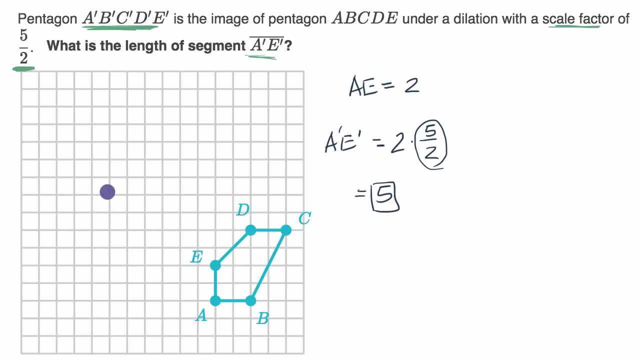 A prime, B prime, C prime, D prime, E prime. In fact, they haven't even given us enough information. I could draw the scale of that, but I actually don't know where to put it, because they didn't even give us our center of dilation. 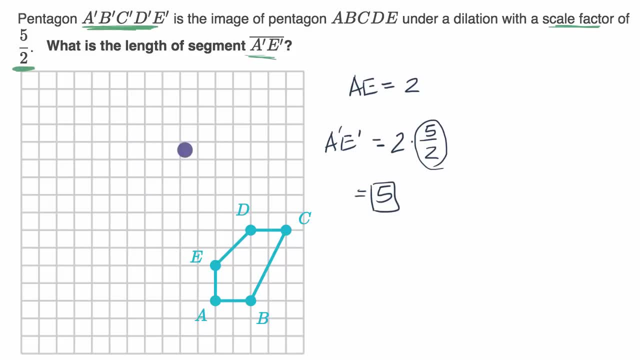 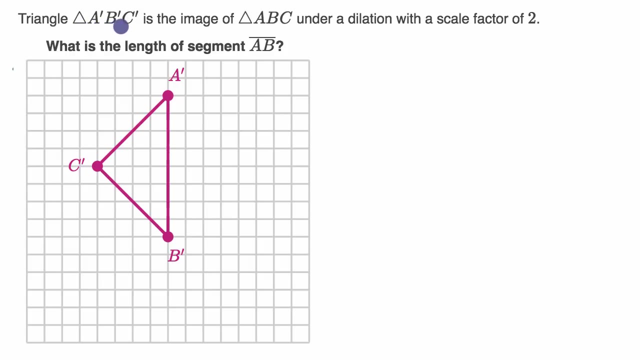 But we know that corresponding sides or the lengths between corresponding points are going to be scaled by the scale factor. Now, with that in mind, let's do another example. So we are told that triangle A prime, B prime, C prime, which they depicted right over here, 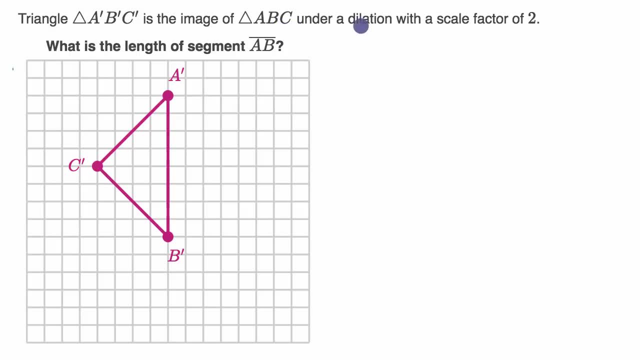 is the image of triangle ABC, which they did not depict under a dilation with a scale factor of two. What is the length of segment AB? Once again, they haven't drawn AB here. How do we figure it out? Well, it's gonna be a similar way as the last example.